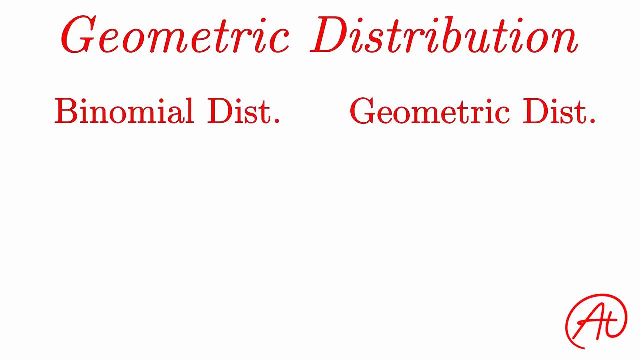 the geometric distribution is really just a more restricted version of the binomial distribution used for a specific scenario. The geometric distribution requires the same conditions to be met as binomial one in order to be used. However, the binomial distribution is used when you're ultimately trying to find the probability of getting a certain number of x. 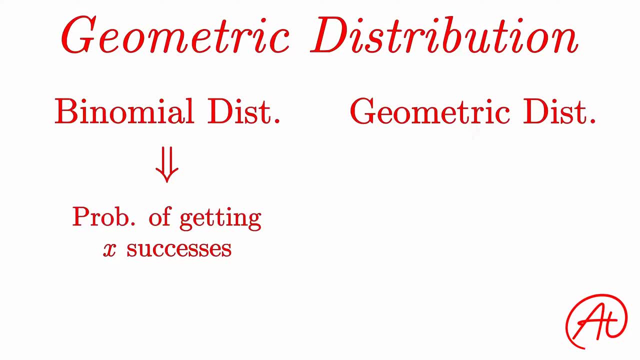 successes out of step xi to a given number x, Then we'll talk about it later- your total number of trials where the geometric distribution is used when you're ultimately trying to find the probability of getting your very first success on a specific trial, number x. 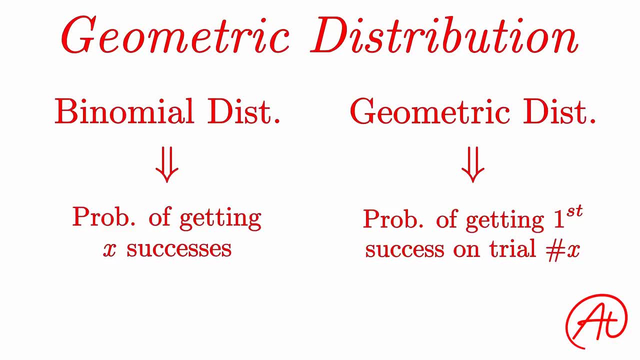 So, for example, you might be a salesman going to sell insurance door to door and you want to find the probability of getting a successful sale on your first house or third house or fifteenth house. Now that we've covered the concept at a high level, let's now go over a couple key parameters. 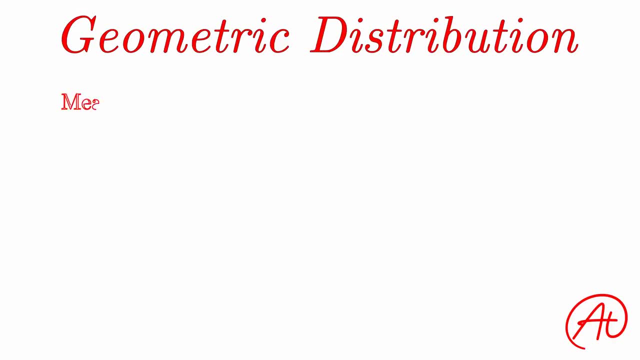 for this distribution. First, the mean, or expected value. This parameter is pretty straightforward and is just: mu equals 1 over p, where p is the probability of getting a success on any given trial. Basically, what the expected value gives you is the amount of trials you can expect to. 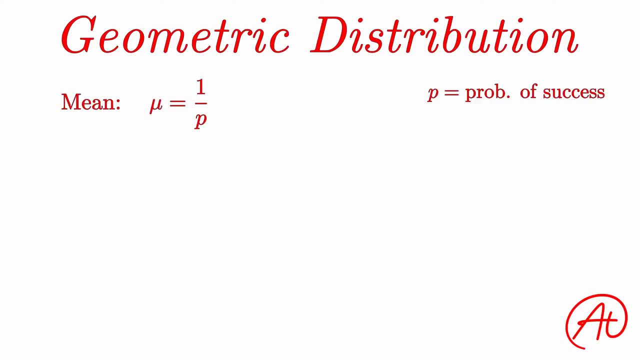 go through before getting your first success, Okay. Next is standard deviation. This value sigma equals the square root of 1 minus p divided by p. or you might see it as the square root of q divided by p, where q just equals 1 minus p, or the probability. 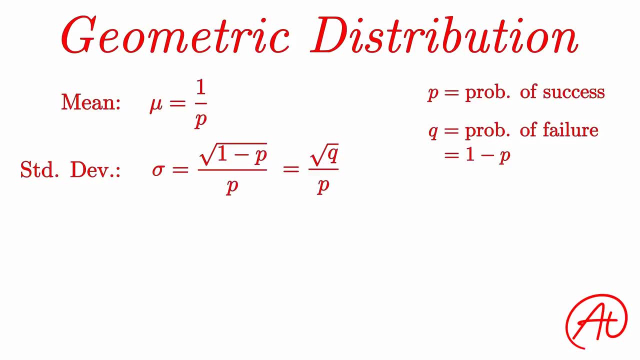 of a failure on any given trial, since there are only two outcomes: a success or a failure. Finally, we have probability and in order to understand this formula, let's take a step back and remember what our scenario looks like For geometric distribution. we want to find the probability of getting our first success. 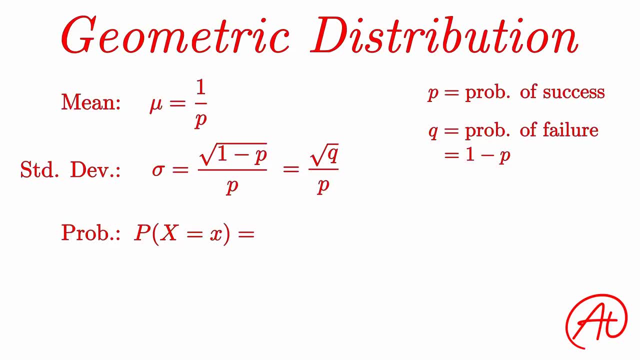 on a certain trial number In order to have our first success on some trial number x. that means that we must have had failures on every trial before trial number x. So if we had this many trials before our first success, we would have had a failure. 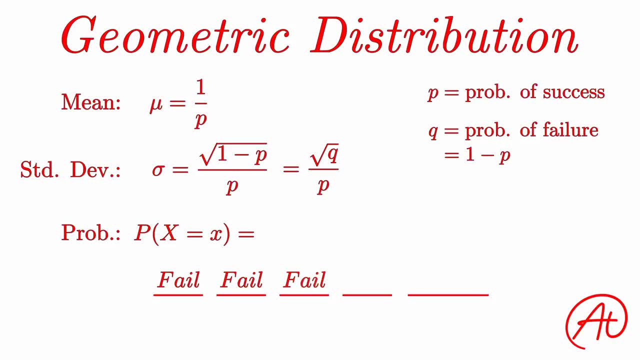 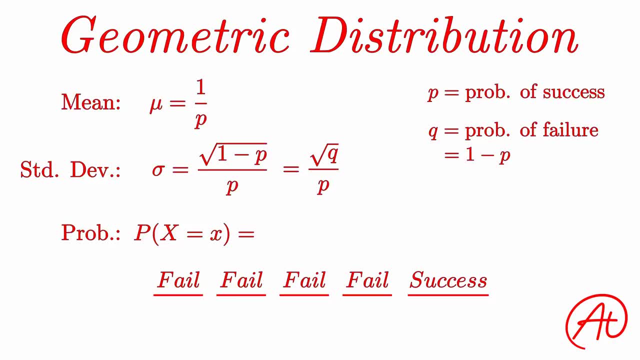 Well, since the same conditions as the binomial distribution must have been met, we know that each of our trials are independent from one another, And when you have independent events, you can simply multiply the probability of each event together to get the overall probability of the events occurring. 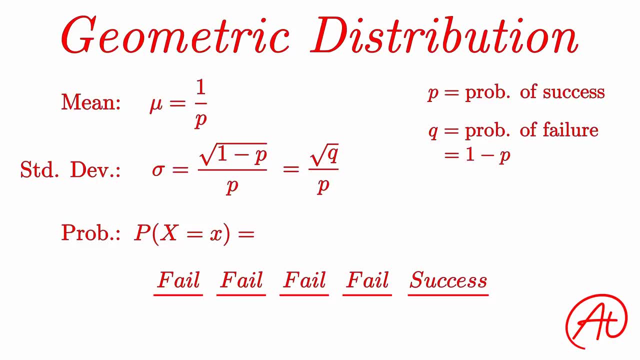 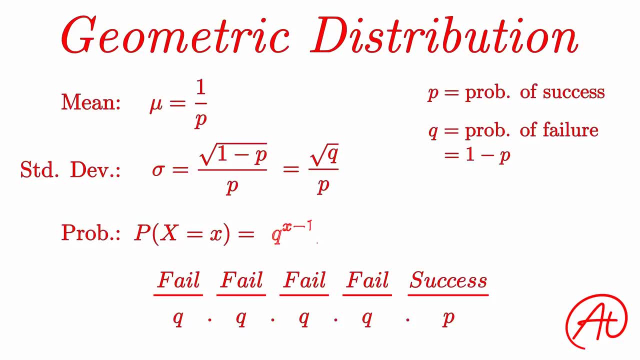 and one success at the end, which reduces to q, raised to the x minus 1 times p, where x again represents the trial we want our first success on. Finally, let's solidify this concept with an example Coming home from work. you always seem to hit every single light. 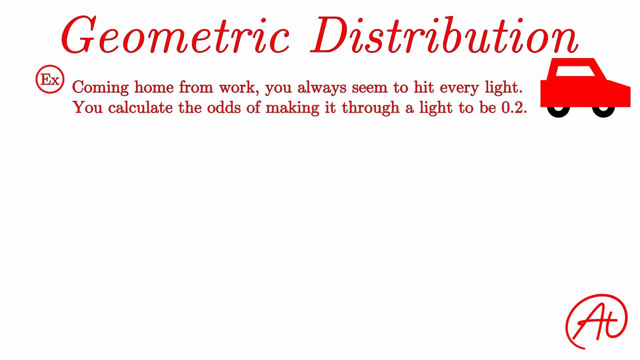 Throughout time. you calculate the odds of making it through any light to be 0.2.. On any given night, how many lights can you expect to hit before finally making it through one, And with what standard deviation? Finally, what's the probability of the third light you come across being the first one? 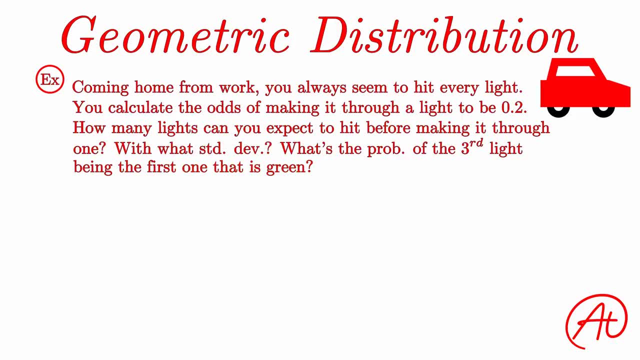 that is green. Okay, this might seem like a lot, so let's unpack it a bit. In this problem, our success is making it through a light without having to stop, And we determined the probability of that occurring to be 0.2, so that's our p-value. 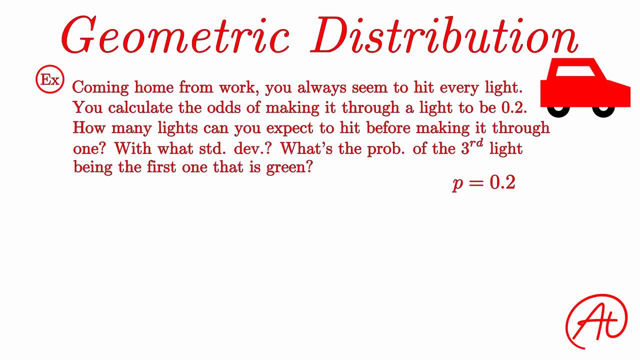 which makes our probability of failure or having to stop at the light equal to 0.8.. Alright, first we want to find out how many red lights we can expect to hit before finally coming across a green one. Okay, so we're going to start with a red light and we're going to start with a green one. 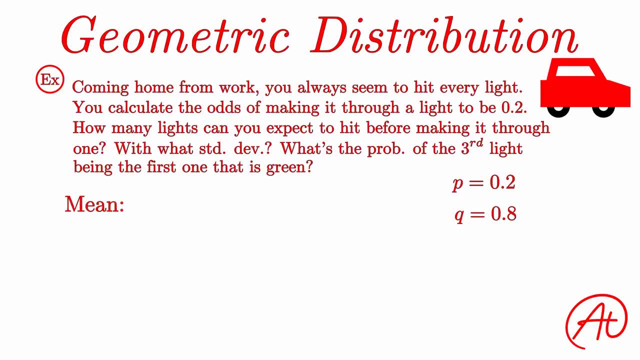 Okay, so we're going to start with a red light and we're going to start with a green one. This is the job for our expected value formula, which states that mu is equal to 1 over p And using our p-value, we get 1 over 0.2, or 5 lights, which means that on any given